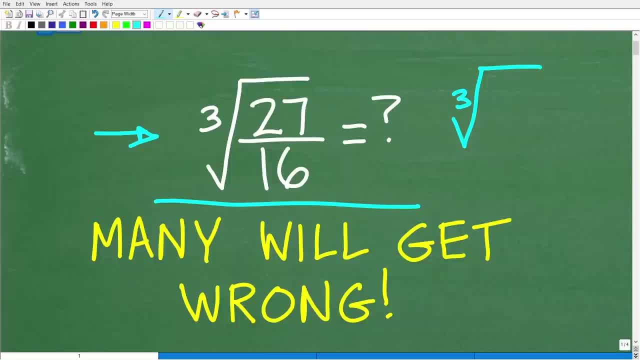 Of course, we can have square roots or, like this problem right here, a cube root or the fifth root, But the properties are the same whether we're dealing with a square root or a cube root. So you want to keep that in mind as you think about this problem. But what we want to do here is simplify. 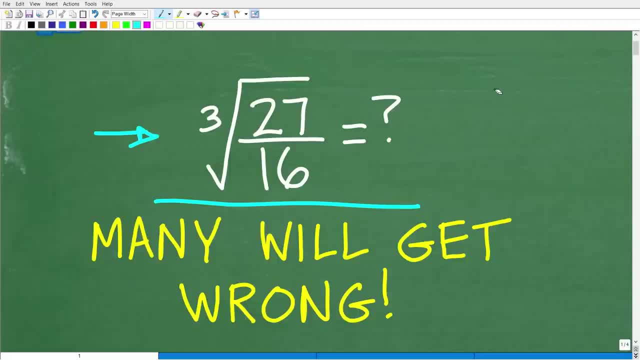 this expression without using a calculator. Now, a lot of you out there probably could do this problem if it was involving only a square root, But because we have a cube right here, this is going to be much more interesting and a lot of you probably are not going to get this right. 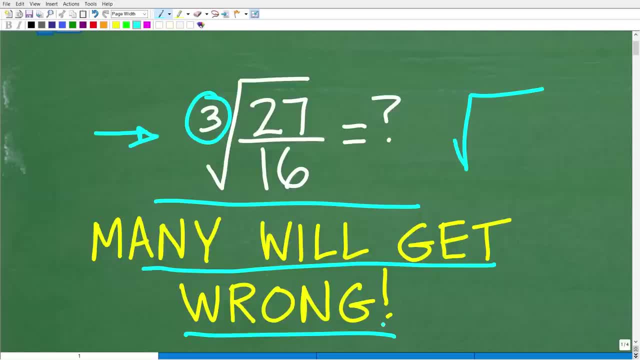 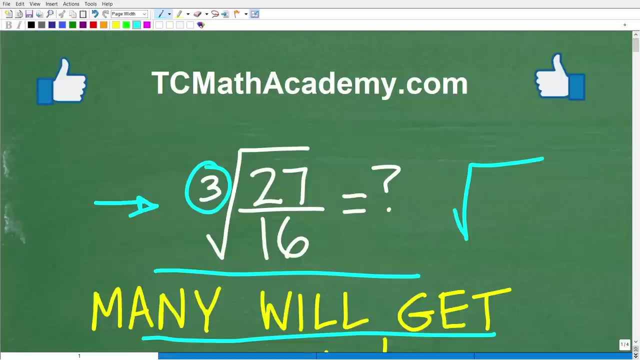 But maybe you are the exception. So if you think you can do this problem again without a calculator, well, go ahead and put your answer into the comment section. I'll show you the correct answer in just one second. Then, of course, we'll walk through exactly how to simplify this expression again. 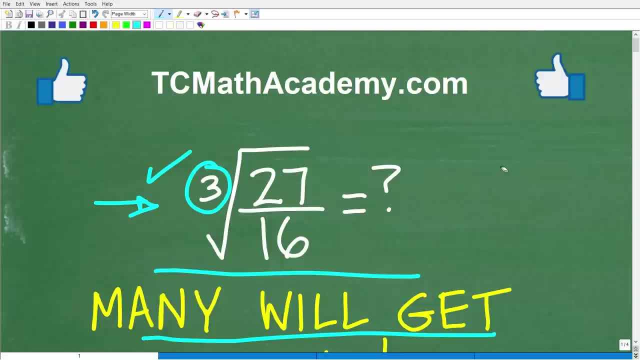 without using a calculator. This is an absolute must-know algebra skill. But before we get started, let me quickly introduce myself. My name is John and I have been teaching middle and high school math for decades, And if you need help learning math, well, check out my math help program at tcmathacademycom. 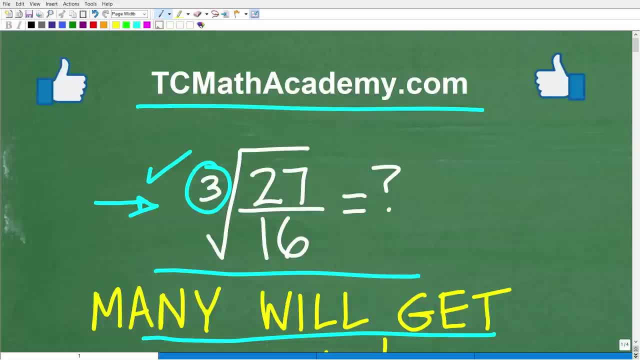 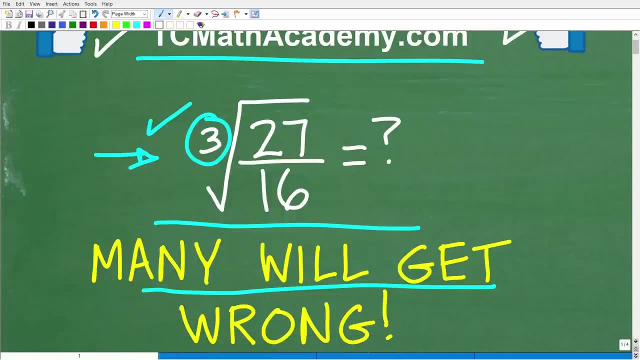 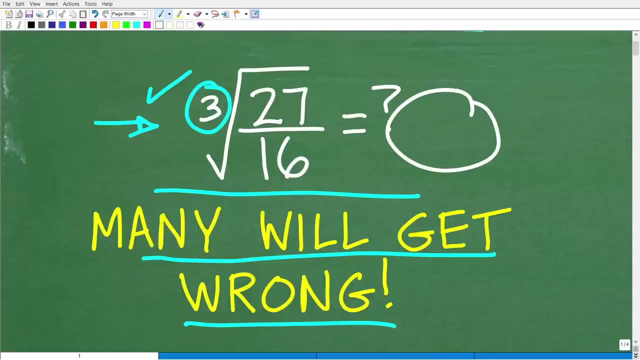 You can find a link to that in the description below, And if this video helps you out, or if you just enjoy this content, make sure to like and subscribe, as that definitely helps me out. Okay, so again we have the cube root of 27 over 16.. We want to write this in its simplest form. 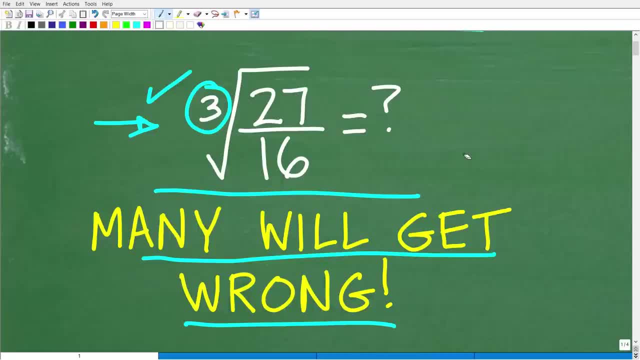 And this is not an optional type of thing in math. Some of you might be saying, hey, Mr YouTube Math Man, you don't even have to fix this up. Well, if you have like, let's say a fraction, 100 over 200. 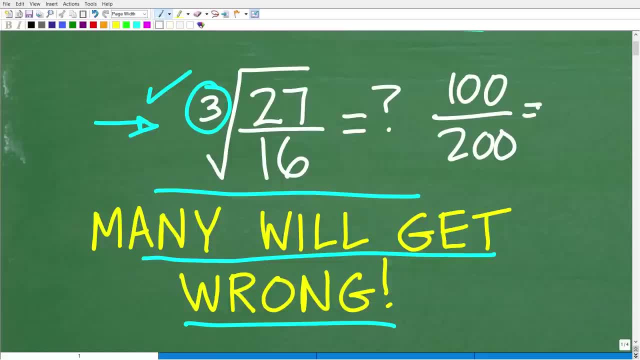 and you gave that to your math teacher, or you answer this on a test that would not be looked upon nicely. Okay, and in mathematics, again, it's not really an optional thing. You must simplify your answer. So in this case it would be one half, So obviously this is a fraction. 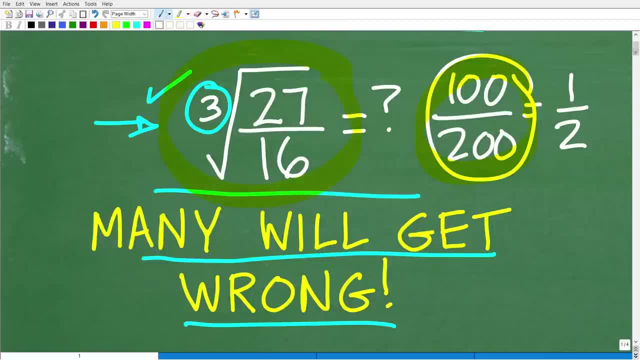 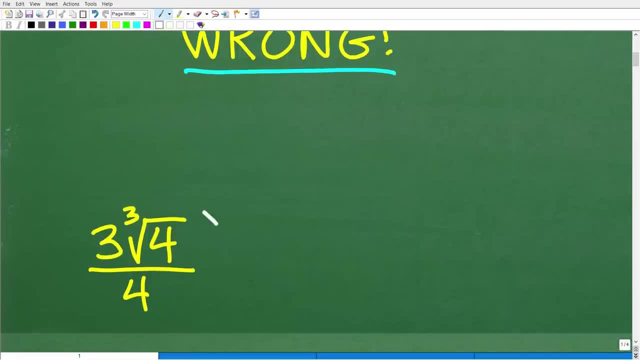 It's pretty easy to simplify. This is much more interesting, And let's go ahead and take a look at the answer. So the correct answer is the following: Three times the cube root of four over four. All right now, if you got this right, that is very. 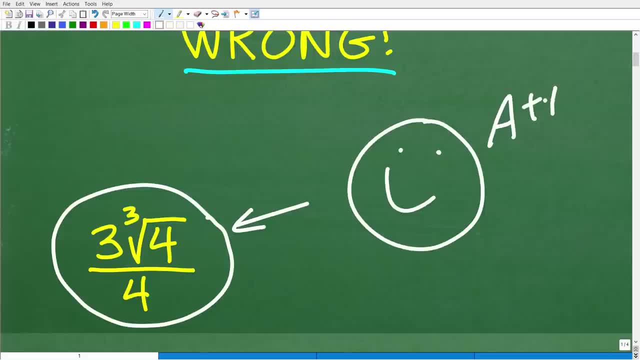 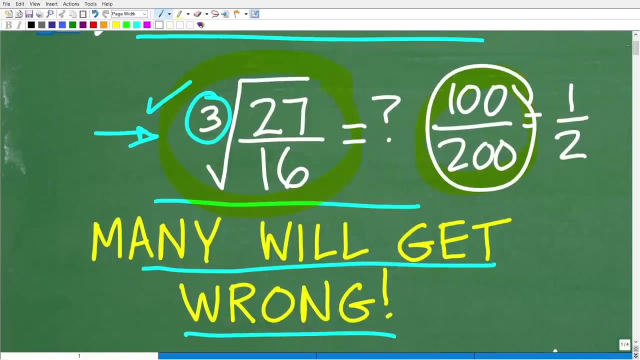 impressive. Matter of fact, I have to give you a nice little happy face and A++. I think I want to give you like 120% and multiple stars so you could tell your friends and family that indeed you are a certified professional expert in the area of simplifying radical expressions. Now, your friends, 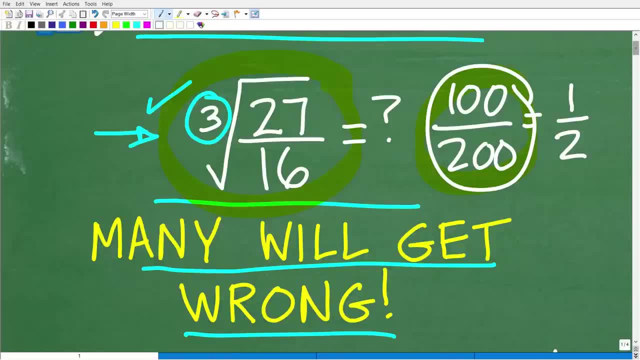 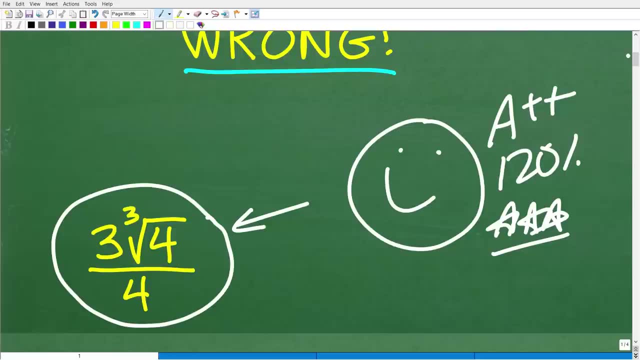 and family won't really understand what that means. but it just sounds pretty impressive to say Now, if you didn't get this right, don't despair, because you probably very well could have been on the right track. But this problem has a bit of a twist, And I don't think a lot of math textbooks 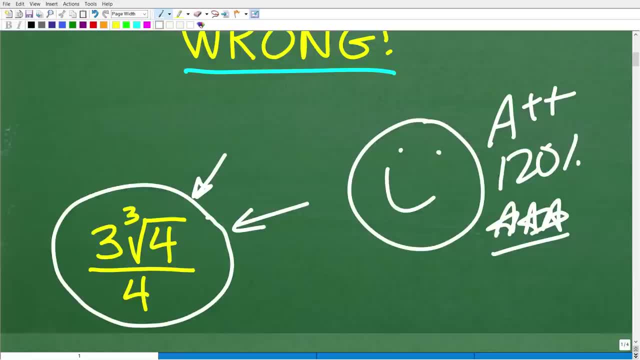 have enough of these type of problems involving cube roots, etc. etc. Well, maybe your class does, or maybe your textbook that you used or are using has these, But anyways, let's go ahead and get into the solution. So, again, what we want to do here is simplify this expression, So let's go ahead. 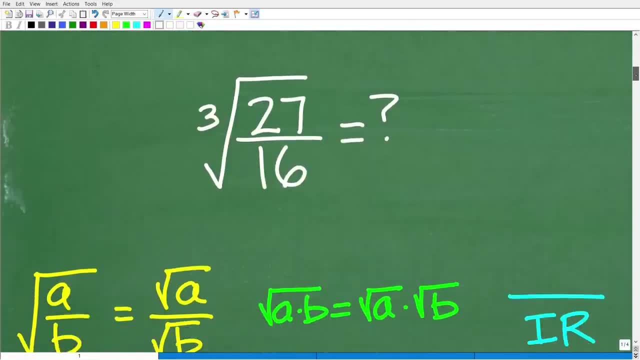 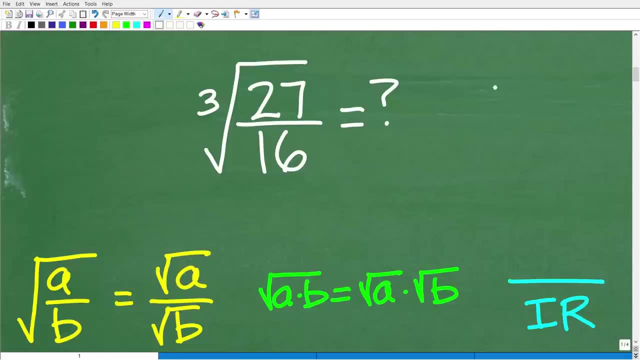 and get into the solution. So, again, what we want to do here is simplify this expression. Now, if you want to simplify this expression without using a calculator, now of course there's going to be times where you're going to want to find the cube root of a number and you need to know how to. 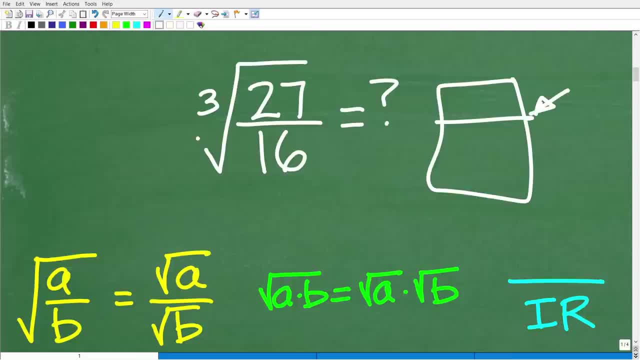 actually use your calculator to do that. So if you wanted to find the cube root of this number, you would take that value of this fraction to the one third power. But that's kind of a separate discussion. But if you're interested in how to find the cube root of numbers or the fifth root, 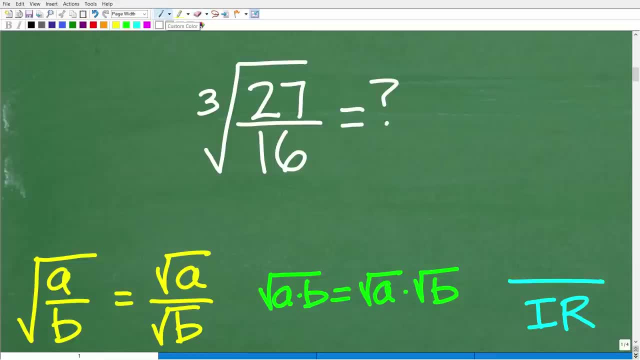 or the seventh root. this is something called rational exponents. But anyways, again a separate topic, But I bring it up because if you wanted to check your work here on a calculator, that's what you would have to do, OK. but in order to do this problem, we need to understand some principles of. 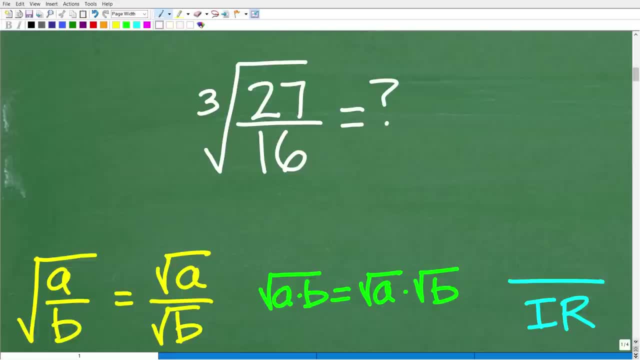 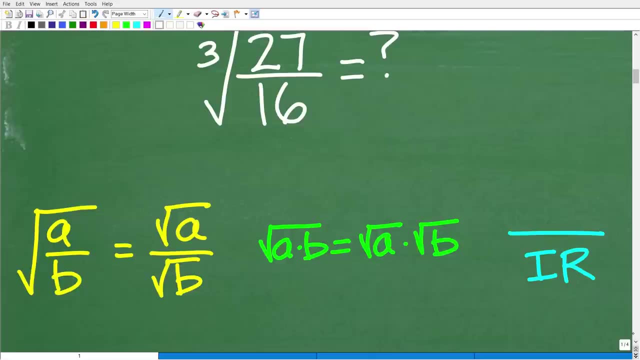 radicals and square roots, And of course you learn these principles when you first start studying square roots And then these problems kind of evolve into more interesting things like cube roots, et cetera, et cetera. OK, so these are the main components or the main properties of radicals. 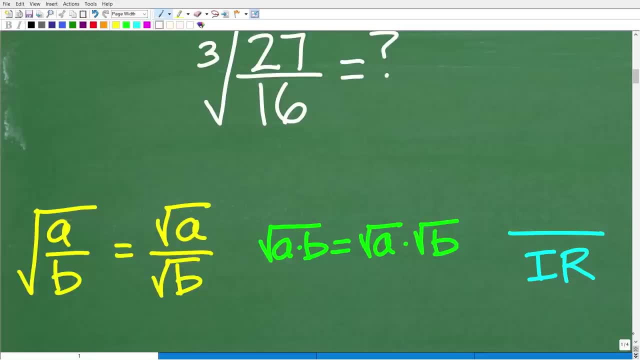 that we need to consider to do this problem right here. So let's go ahead and get into the solution And hopefully you know you're looking at these things, you know make sense to you. Maybe this one right here is a little confusing, So I'm just going to quickly go over these right now. All 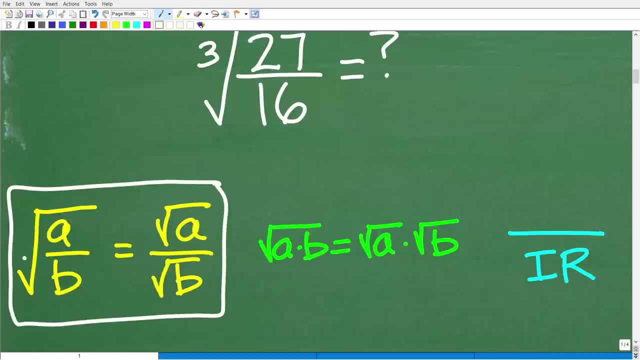 right. So our first property is the following: When we have the square root or a radical of a fraction, we can actually break this up into two individual square roots or radicals. So the square root of A over B is equal to the square root of A over the square root of B. We will be using this. 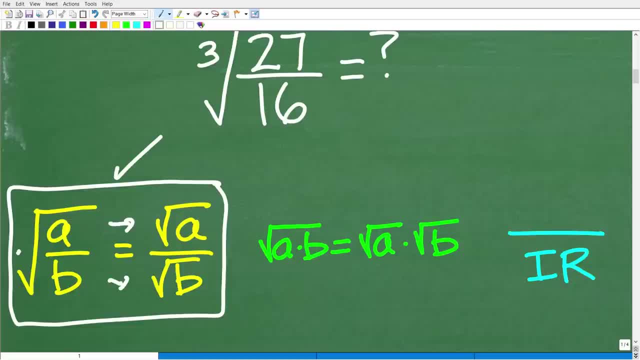 in this problem. OK, now, of course, we're going to have to do this problem. We're going to have to. this is the square root, but it could be the cube root as well, or the fifth root. Just everything has to be cube roots or fifth roots or whatever the case might be. All right, Same thing applies, right. 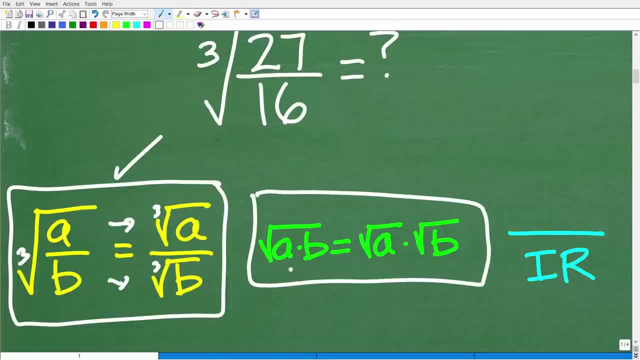 here that the square root of a number And if you can look at this number or value in terms of its factors, So the square root of A times B is equal to the square root of A times the square root of B. So we can break this up and we can just find the square roots of the radicals of the individual. 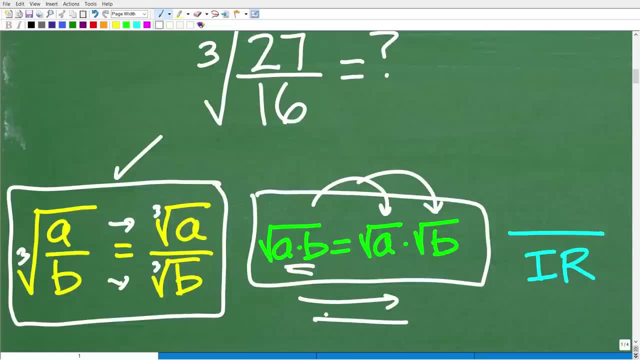 factors. OK, so this property goes this way and this way. Likewise, this property goes this way and this way. All right, So hopefully all of this makes sense to you. And the last thing here is the following: So you cannot leave your answer with an irrational number in the denominator. So let's suppose I had like seven. 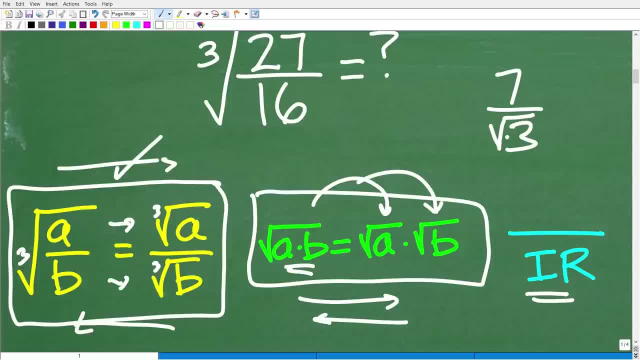 over the square root of three And you're like I'm going to turn this into my math teacher. I would say no, no, don't do that. That's not good, because right down here in the denominator we have an irrational number. OK, so the square root of three is irrational. Now, if you had like, 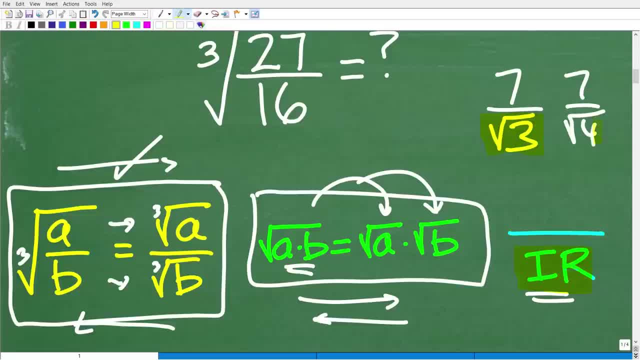 seven over the square root of four. this is not a problem, because the square root of four, of course, is two, which is rational. OK. but we can't have, we can't leave our final answer with a irrational number in the denominator. So we have to fix this up. So a quick review: How do we fix this problem? 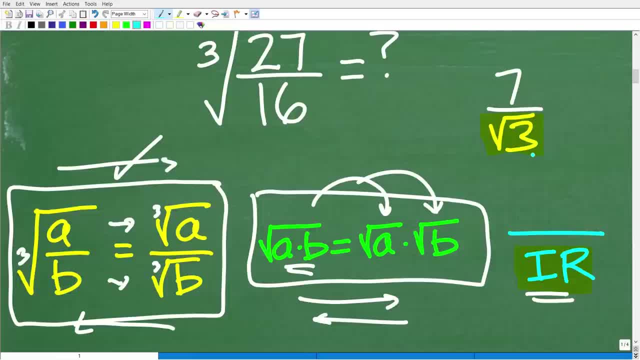 right here. Well, we do something called rationalizing the denominator. So we're going to multiply both the denominator and the numerator by the square root of three, And we're going to- and it would fix this up, And of course we'd have the square root of three times the square root of. 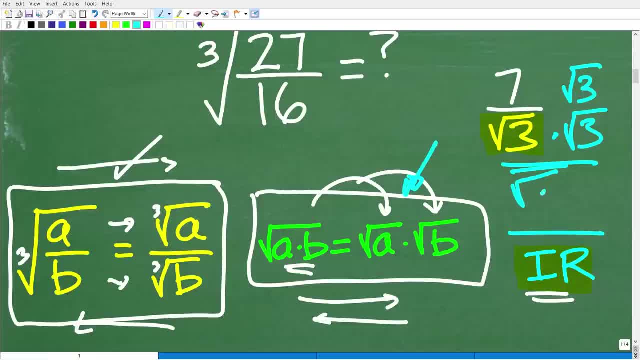 three. We'd be thinking about this property here. which is what? Well, that's the square root of nine or three. So this would be seven times the square root of three over three. All right, Now, if you understand all of this, you're saying: yes, Mr YouTube, math man, I get what you're saying. 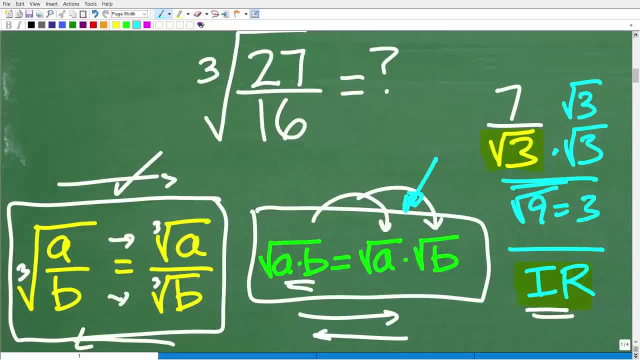 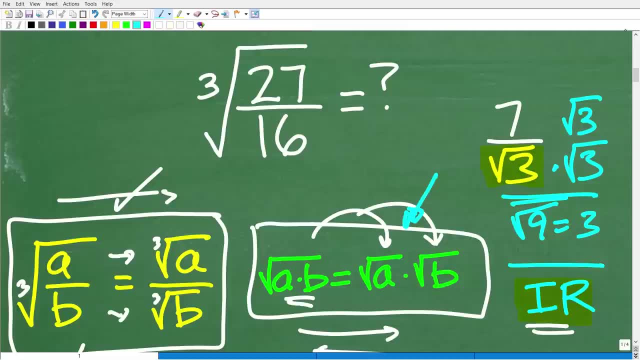 Well, these are the hints. These are the considerations that you need to be thinking about in order to do this problem right here. OK, so if you didn't remember these properties and you maybe want to give this problem another try, we'll pause the video and give another try, But we're going to go ahead and get into this right. 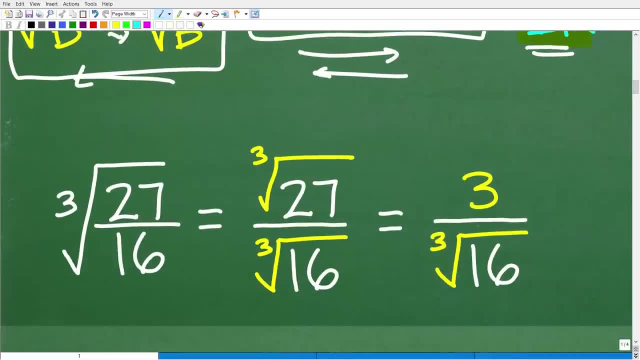 now, OK, so first things first. I have the cube root of the square root of twenty seven over sixteen. So I'm going to go ahead and break this up into two individual cube roots. Right, So we're dealing with the cube root, not the square root, but it works the same way. So one big radical I could. 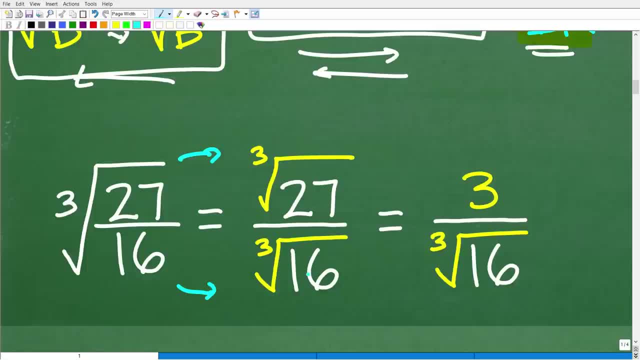 break it up into the a radical of the numerator and a radical of the denominator. Of course, we're dealing with cube roots here. Now, this is fantastic because the cube root of twenty seven is what It's three, Remember. the cube root is asking the question what number times itself gets back to this number. 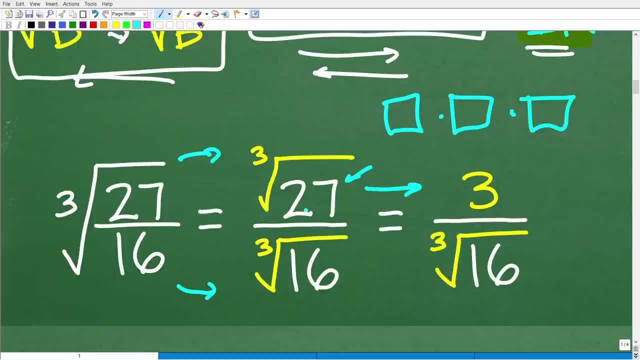 OK, so what times itself? three times gets back to twenty seven. It is three. So three times three times three is twenty seven. So the cube root of twenty seven is three. All right, So hopefully most of you are with me at this point and you're saying yes, Mr. 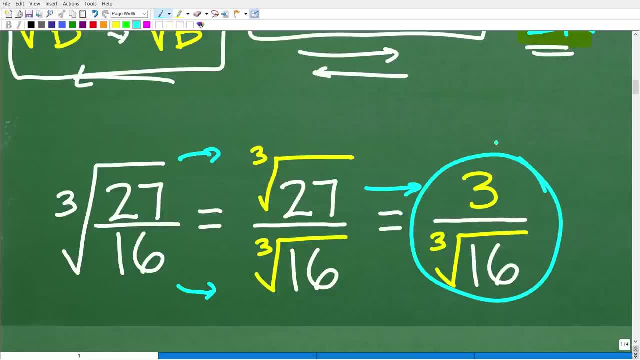 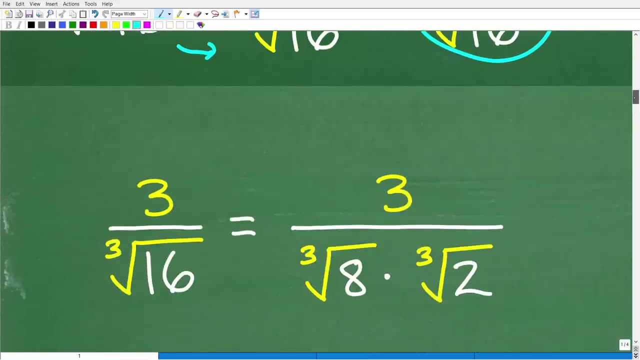 YouTube math man, I see where you're going with this. Well, this is pretty good and we have a good start here, but certainly our denominator needs some work. But we can fix that- the cube root of sixteen- by thinking about this property right here. OK, so let's go ahead and get into that right now. So we have three over. 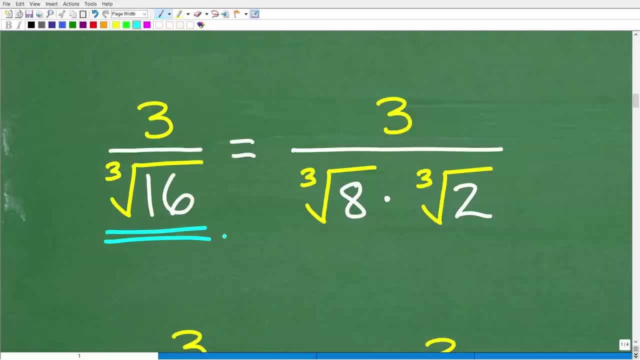 the cube root of sixteen. So obviously we can't leave our answer like this, But what we can do is break up sixteen into its factors, Right? So you want to be thinking of factors, as we were saying. So you have four times four. Now, this is OK, These are perfect square. 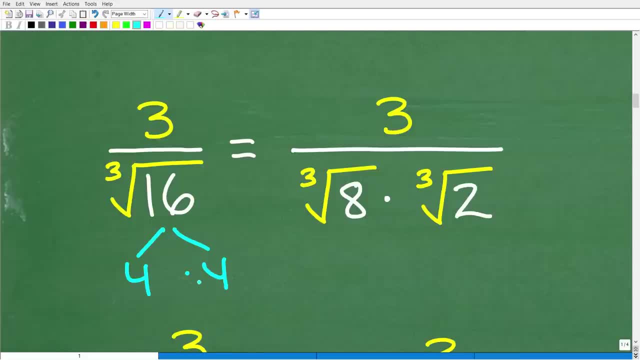 factors. This would be great if we were dealing with square roots, but we need to be kind of thinking in terms of cube roots. So four and four is not going to really help us out, But eight and two would help us out because we know the cube root of eight. So this is. 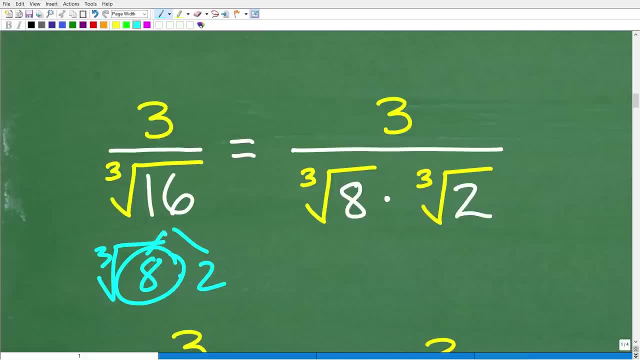 kind of the main idea, And a lot of you, I think, are probably pretty good at these problems when they're only kind of square roots. But if you're thinking of the cube root, you're going to have to kind of think, you know. 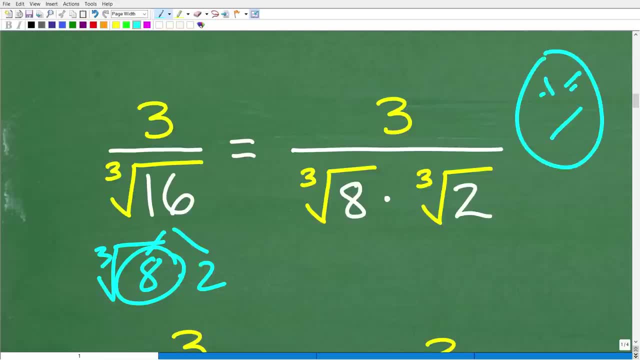 in your brain. you're going to have to be like: all right, I love drawing pictures. If you've seen my videos, you can know I just have fun with this stuff. All right, So you have to switch from this to the cube root in your brain. You have to make that leap. 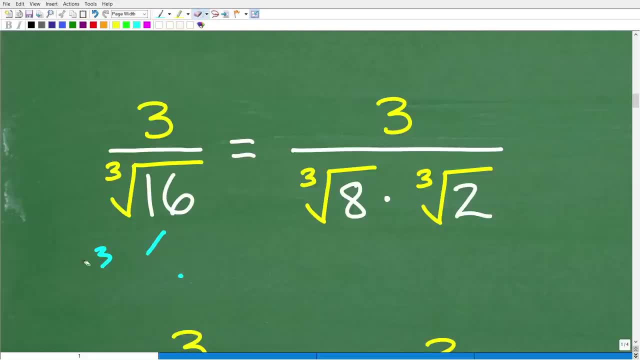 here, because if you're stuck on square root you're not going to be able to see the right solutions here. So for sixteen, I want to break sixteen into the factors of eight and two. OK, so we can write this as the cube root of eight, And then we're going to have 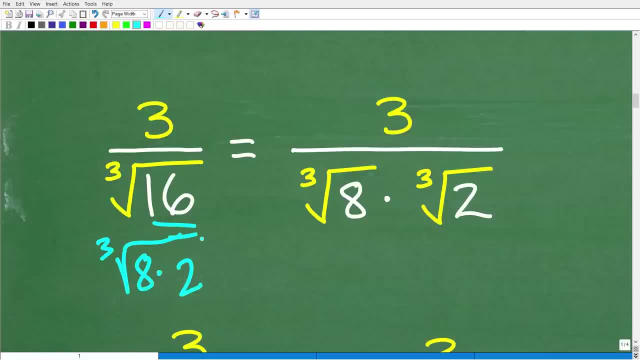 the cube root of eight times two. Now I can break this up into its component parts. So the cube root of eight, And I like this because I know what the cube root of eight is. So what number times itself is eight. You might be saying, well, that's two, Mr YouTube Math. 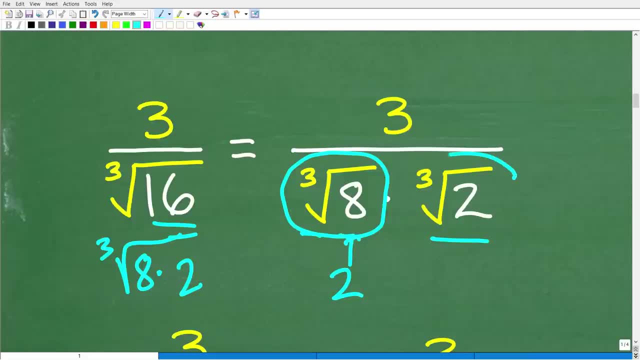 Man, And you would be correct. So we have the cube root of eight times the cube root of two. And you know, we're just kind of whittling this problem down one step at a time, making it a little bit simpler and simpler. OK, so we have three over the cube root of. 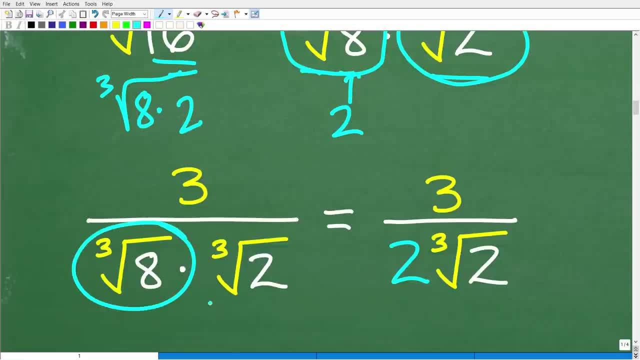 eight, Eight times the cube root of two. Of course this is the cube root of sixteen. So this right here is two. The cube root of eight is two. So now we have two times the cube root of two, or three over, two times the cube root of two. Excuse me, Boy, I'm all over. 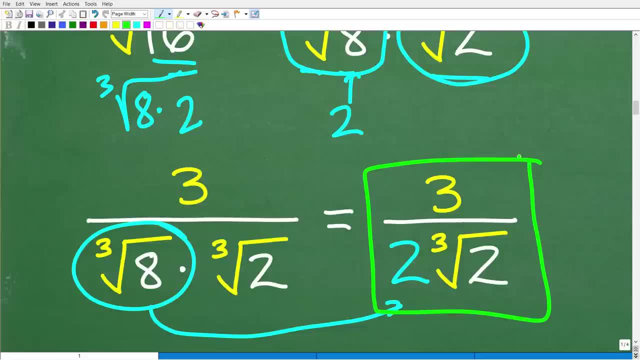 the place here, OK. so this is where we're at and we're making good progress, But we have a problem, OK, and our problem is right here. We still have an irrational number that we have to get rid of, So we have to get rid of that, And we have to get rid of that. 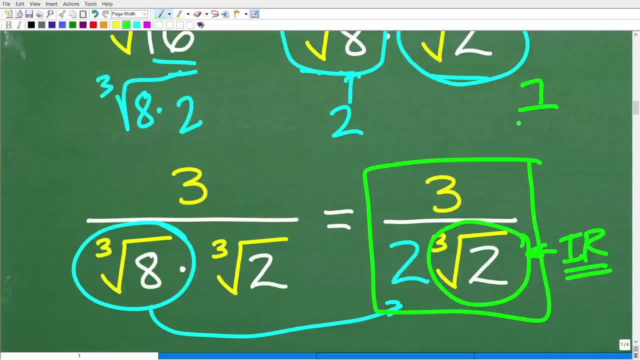 OK. so in this case we're kind of at this point in the problem: seven over the square root of three. So how can we get rid of this square root of three? Well, we just kind of went over that. We multiplied this fraction right here: seven over the square root of. 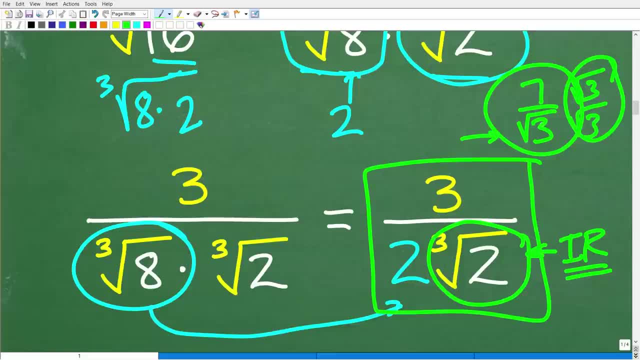 three by square root of three over the square root of three, And it fixed the problem Again. this is called rationalizing the denominator, And most of you are familiar with this when you work with square roots, But this is a little bit different. OK, so let's go ahead. 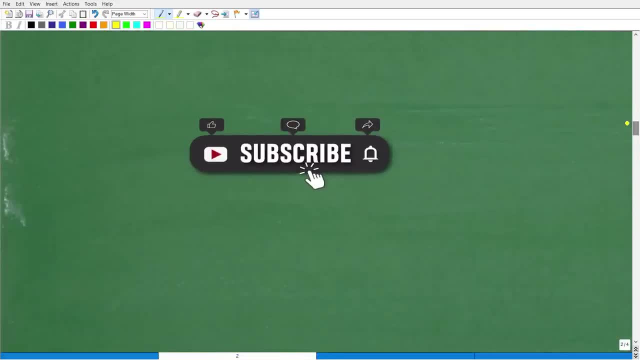 and take the next step, Which, of course, is having you quickly subscribe to my YouTube channel. Now, if you are new to my YouTube channel, I want to welcome you. Thank you so much for dropping in, And just a little bit about myself. I've been teaching math, as I said in my intro, for a long long. 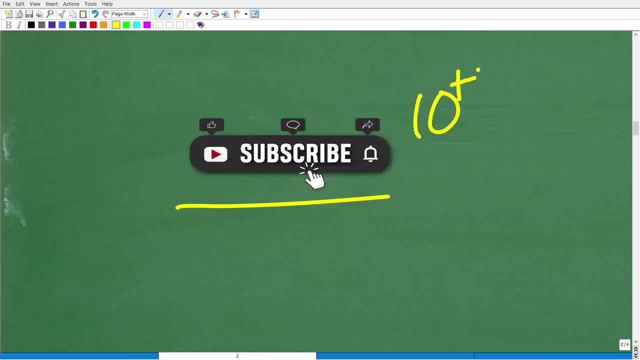 long time, But I've been on YouTube for quite a while, well over 10 years. I have well over 2,500 videos, from basic math to advanced math by calculus and everything in between. My kind of main mission on my YouTube channel is to make sure that I'm able to help you. 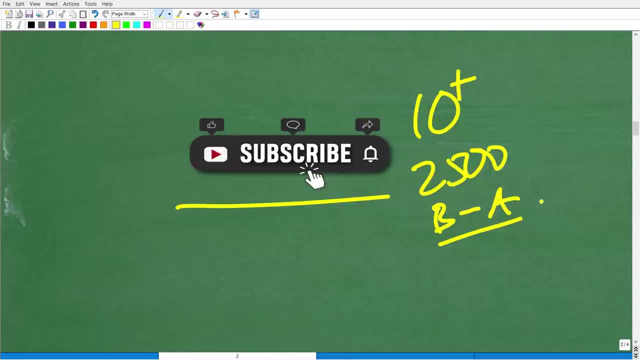 make math clear and understandable, right? Especially, there's so many people out there that you know their math confidence is pretty low. They're like: I'm bad at math, I don't get math. Well, it's all of this right here. You know, a huge amount of it is not your. 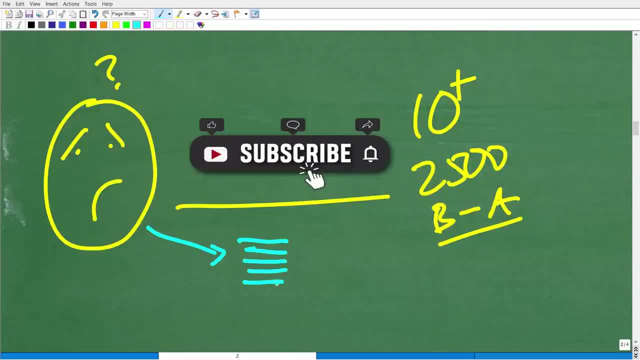 fault if you're in this position. Oftentimes you know we just get a lot of instruction, that you know. I'm not trying to knock any teachers out there, But you know one teacher has a responsibility of teaching a lot of people, So you may not connect with that particular. 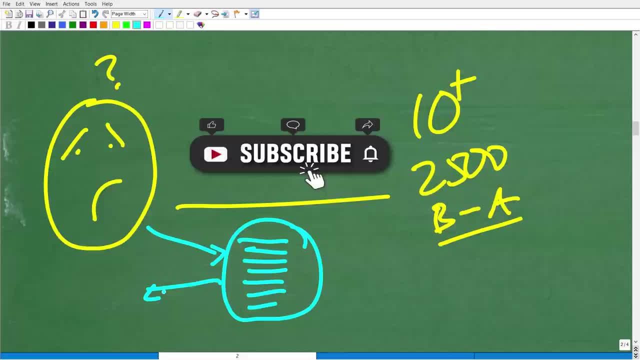 teacher. So that kind of leaves you on your own to figure things out. Now, the first thing you should do is ask your teacher for help, okay, But if that's not working for you, you need to take the initiative and go beyond the classroom, right? So find a teacher that you like and 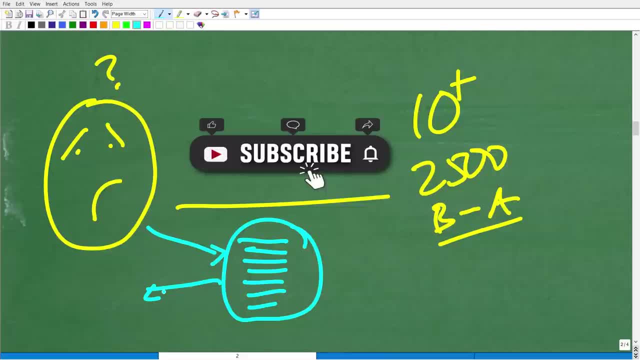 understand that really gives you or can deliver comprehensive math instruction. okay, And that's what I'm all about. I like to break things down piece by piece by piece so everybody gets what's going on. So if you need help with math, okay, whether it's you know a. 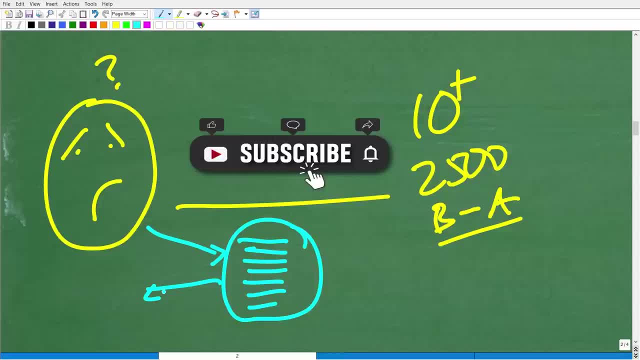 cube root, square roots, radicals, algebra, trigonometry, precalculus. whatever the case is, check out all my courses. I'm going to leave links to them in the description of this video and you can get some follow-on help on this. 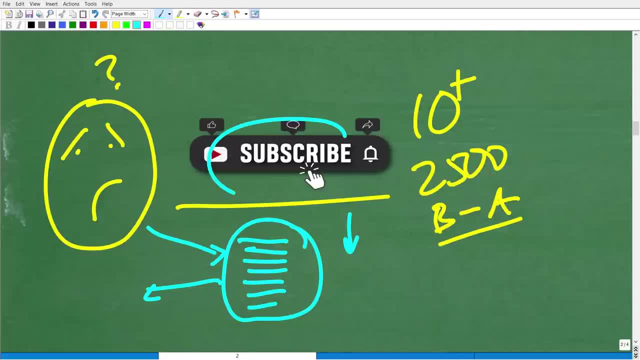 But before we do anything and move on for the rest of this problem, hit that subscribe button, because that definitely helps me reach more people And you know we're kind of both helping each other out. Maybe you're getting some from this video, but you're also 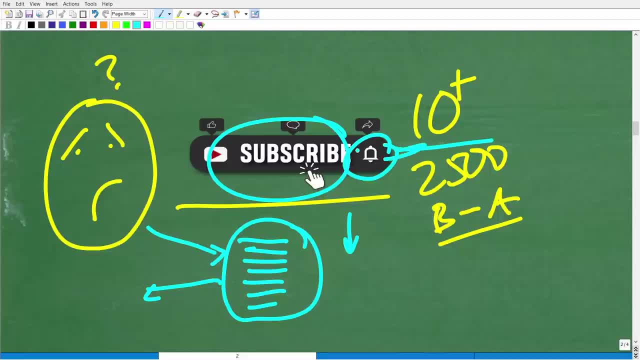 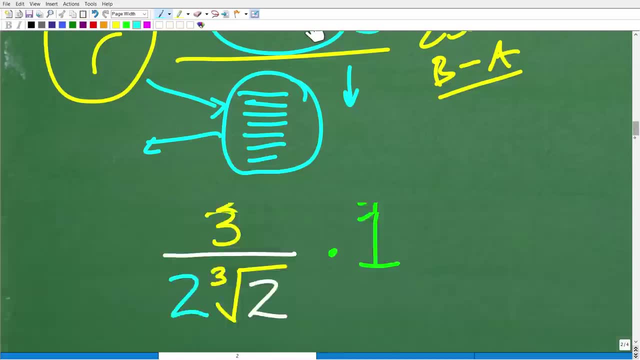 helping me out. So hit that subscribe button And if you're going to do that, hit that notification bell as well, so you can get my latest videos. And thank you so much for giving me a little bit of time to explain what I do. Okay, so now let's get back to this problem now, because 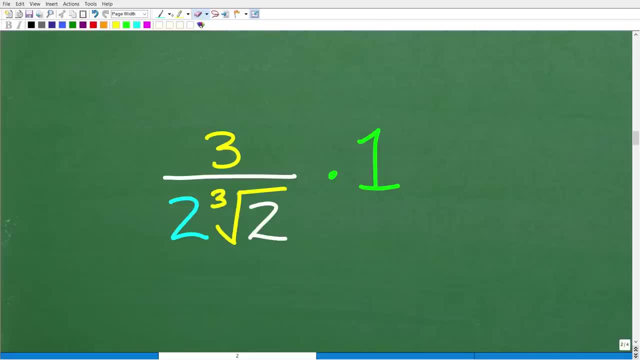 we are not done All right, so we've made some good progress and I think most of you are like: okay, I understand, Mr YouTube, Math Man, you know all the steps up to here. So now we need to fix this fraction up, We need to fix this expression up, And the goal is: 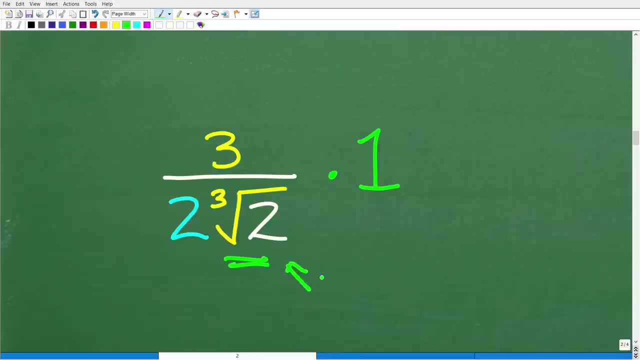 to get rid of this irrational number in the denominator. I don't care if I have one up in the numerator, it's okay, but I can't have it down in the denominator. So the trick that we're going to use is we're going to multiply by one. 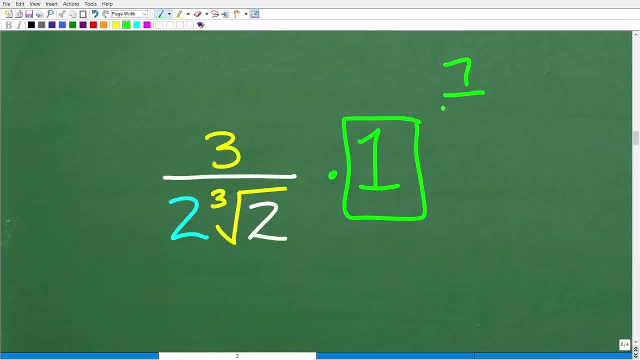 Okay, now let's go back to this little problem that I was doing earlier in the video. seven over the square root of three. Remember, I multiplied both the denominator and the numerator by the square root of three. Okay now, hopefully all of you out there you know are familiar. 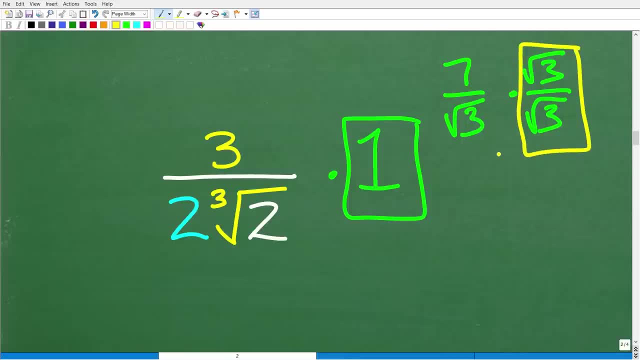 with what I'm doing right in this step, because if you're not familiar with this, well, this particular problem is going to be quite confusing. So let's go ahead and do that. So let's go ahead and do that now. What is this square root of three? over the square root of three? Well, anything divided. 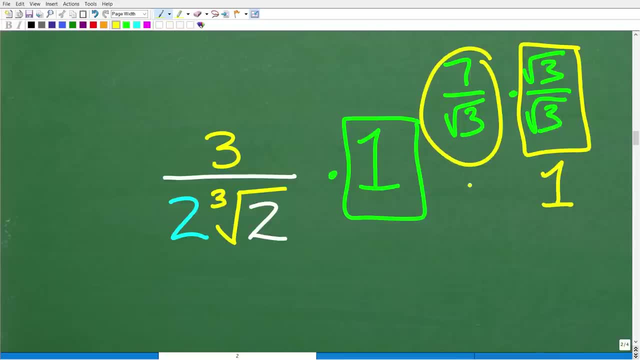 by itself is one. So we're just multiplying this by once. We're not changing the value. Okay, we're rewriting the problem so it looks different, And the objective is again to get rid of those irrational numbers in the denominator Right. so again, the main idea. 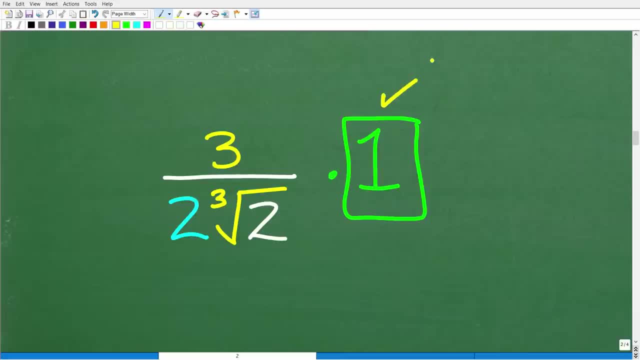 is to think about. what expression can we think of that has a value of one such that we multiply by this. Okay, get rid of this cube root expression down here in the denominator. So I'm going to give you a bit of a hint. okay, You want to be thinking about this right here. numbers that you know: the cube. 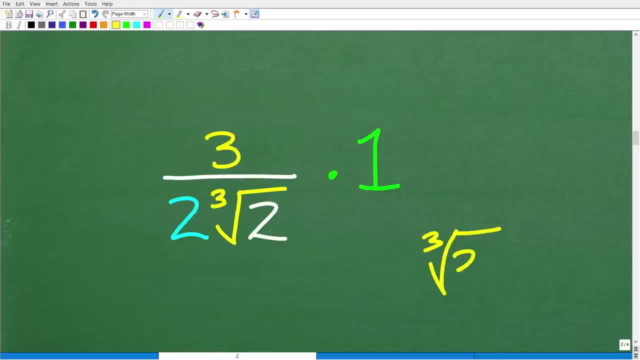 root of right. So what numbers do we know? the cube root of? Well, we know the cube root of 27,, for example, which is 3,, and we know the cube root of 8, which, of course, we know is 2.. Now, 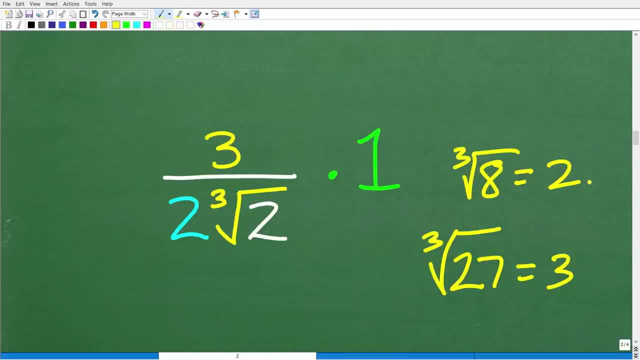 there's other examples we could use as well, but one of these values is what we want to be thinking about in terms of simplifying this expression right here. Okay, so this is just a bit of a clue for those of you that want to kind of follow along or try to do this, you know. 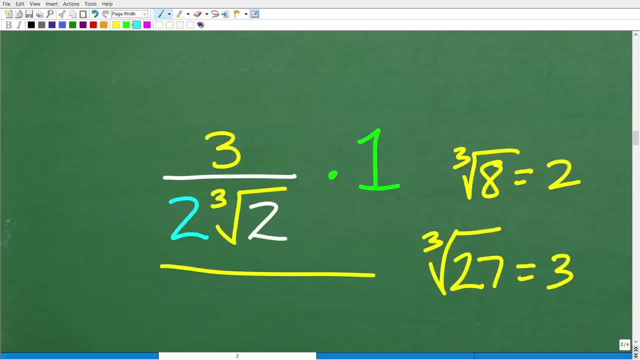 as I actually do it. Okay, so if you're thinking about this- hopefully this is what you are thinking- You're like: hey, maybe we could turn this thing into this thing. and if you're thinking in those terms, well, you are thinking right, Okay, so that's exactly what we're going to do. 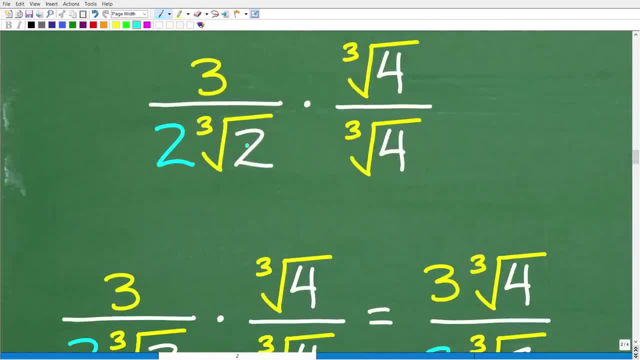 What we want to do. we need to get a cube root situation in the denominator that we know the answer of. So if you know we could turn this cube root of 2 into a cube root of 8, well then, I know the cube root of 8, that is going to be 2.. So let's go ahead and do that. okay, It's not a 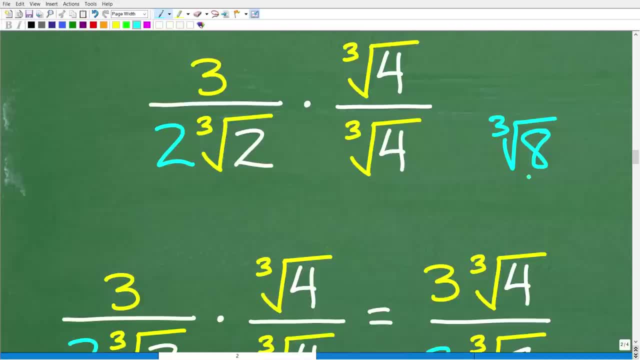 problem here. So how can I turn a cube root of 2 into a cube root of 8? Easy, just multiply this thing by the cube root of 4, right, Because 2 times 2 is going to be 2, and that's going to be. 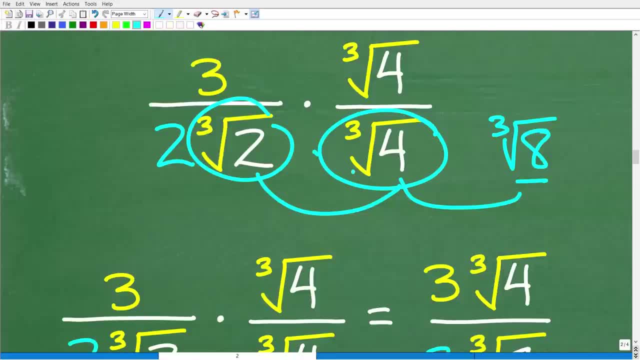 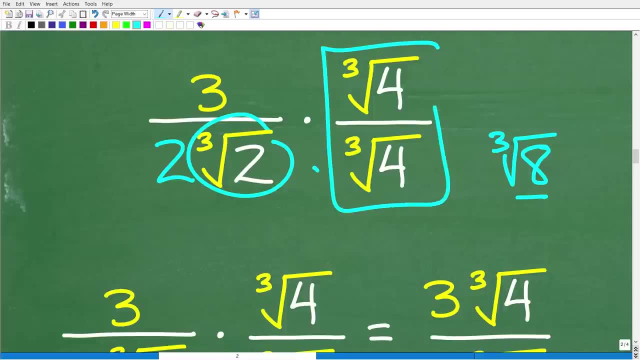 4 times 4 is 8.. So if I multiply the denominator by the cube root of 4, I've got to multiply the numerator by the cube root of 4, because, again, keep in mind that this right here is just a fancy. 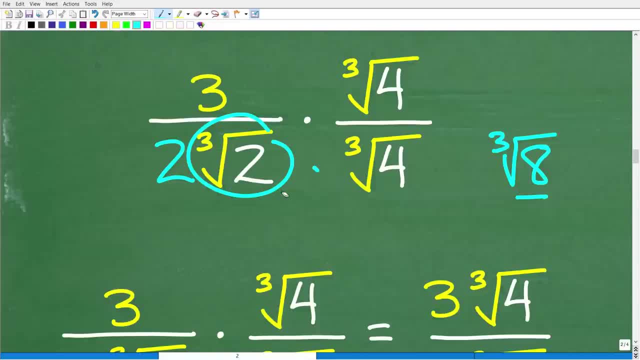 1. It's this thing, divided by itself, which is 1.. Okay, so this is the main trick, and this is probably the most difficult- I don't want to say the most difficult- part of the problem, but this is the part of the problem that I think a lot of people may have struggled with. Okay, so if you 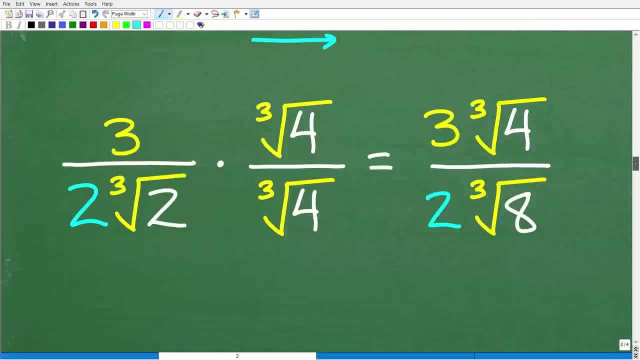 understand this. let's actually go ahead and do the math right now. Okay, so let's focus in on the denominator again. So we have 2 times the cube root of 2, and we're going to multiply this times the cube root of 4, so we can end up with the cube root. 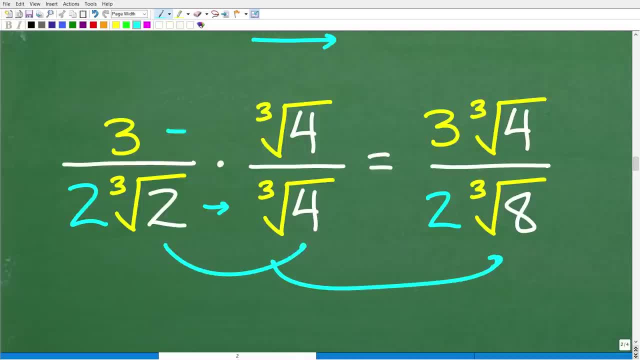 of 8.. So this would be 2 times the cube root of 8, and then our numerator will be 3 times the cube root of 4.. All right, so 2 times the cube root of 8,, again the cube root of 8, pretty. 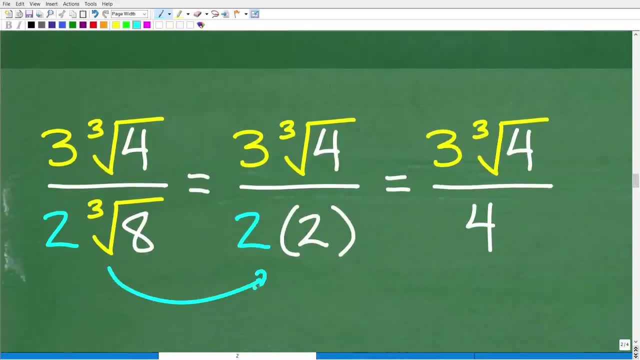 straightforward stuff that is going to be equal to 2.. So I have 3 times the cube root of 4, over 2 times 2, because this is 2, so that's 2 times 2, which of course is 4, and here is our.